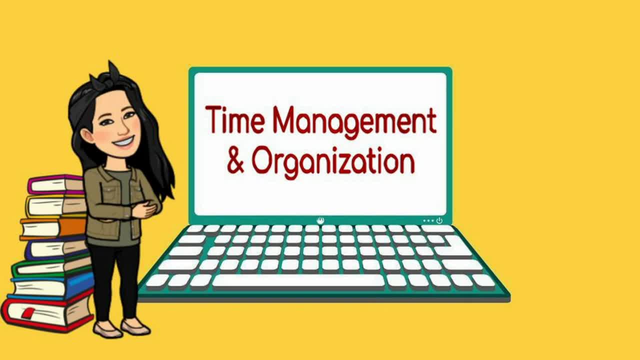 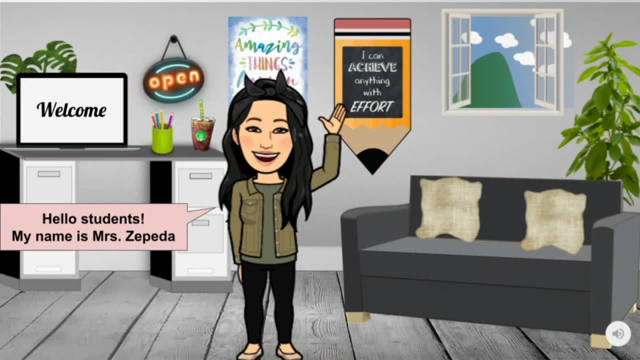 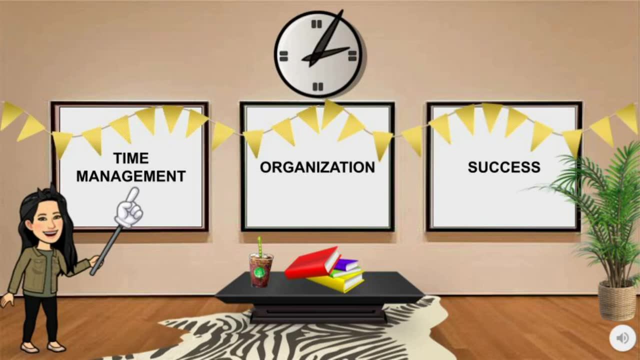 Hello students, welcome. My name is Mrs Cepeda and I am thrilled to talk to you today about important skills you will utilize throughout your life. Today we will discuss time management organization and how this helps us succeed personally and academically. 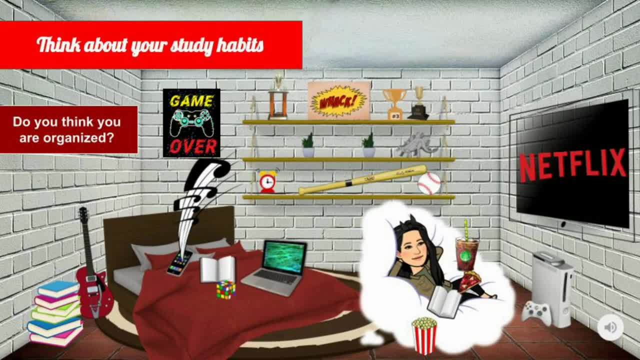 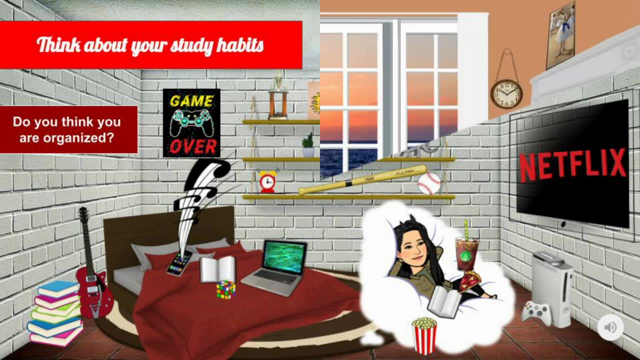 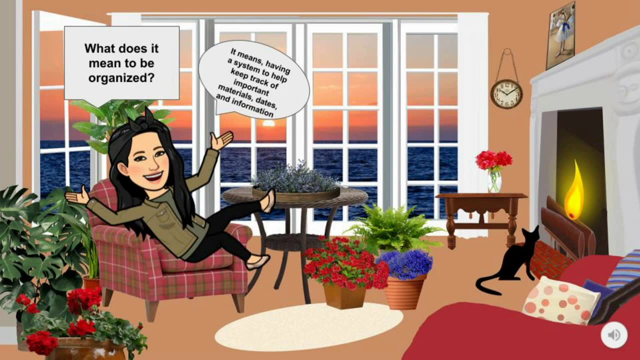 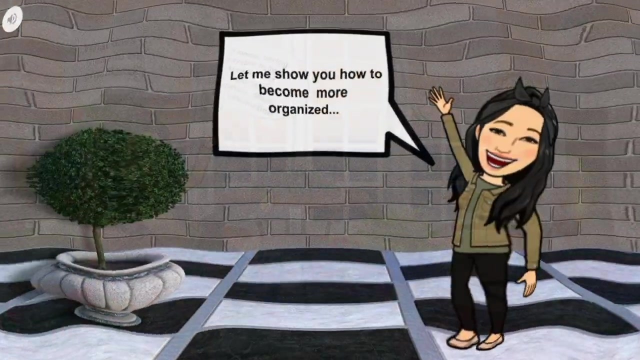 Before we begin, I want you to think about your study habits. Does this look familiar to you? Do you think you are organized? What do you think it means to be organized? To be organized means having a system to keep track of important materials, dates and information. Today, 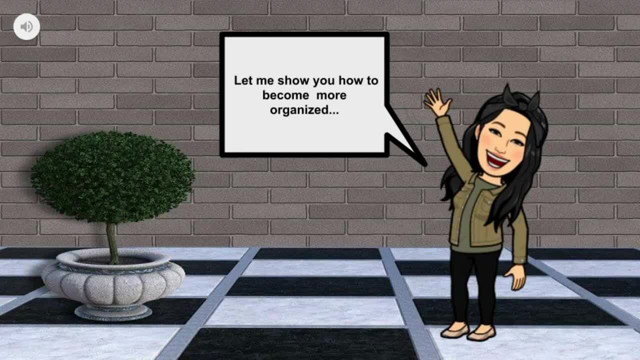 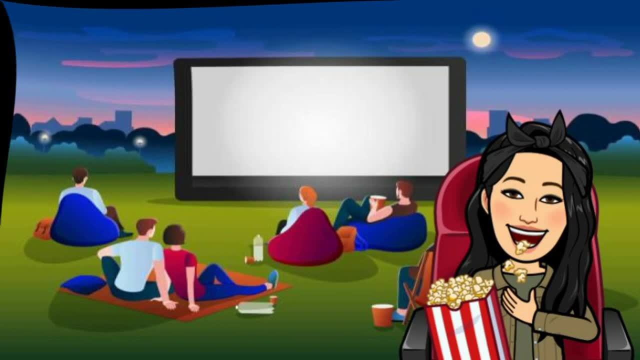 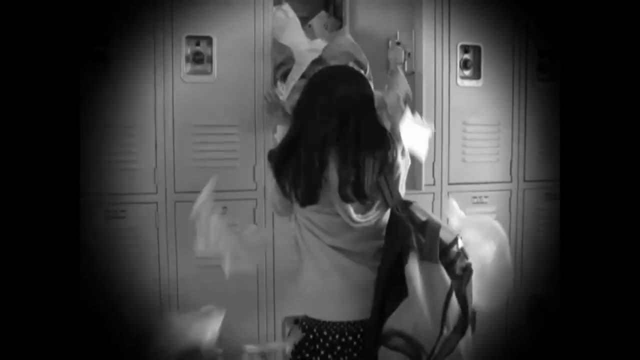 I'm excited to teach you some ways that you can become more organized, But first let's watch a short clip on how being disorganized makes us feel. This girl's science project is due today, But she can't find it in her messy locker. That's an F for you. 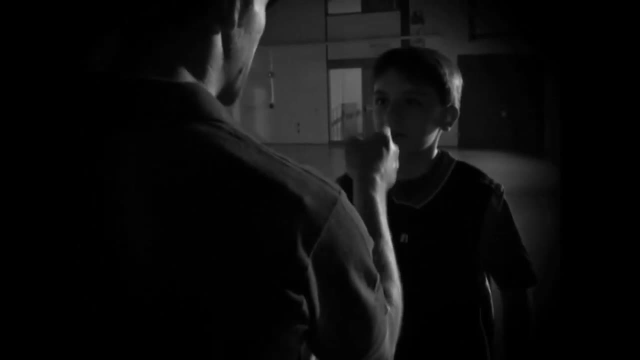 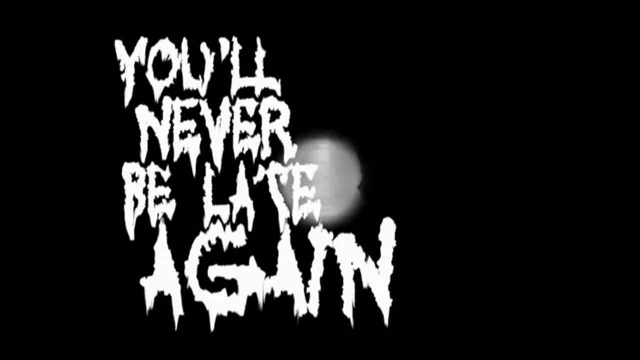 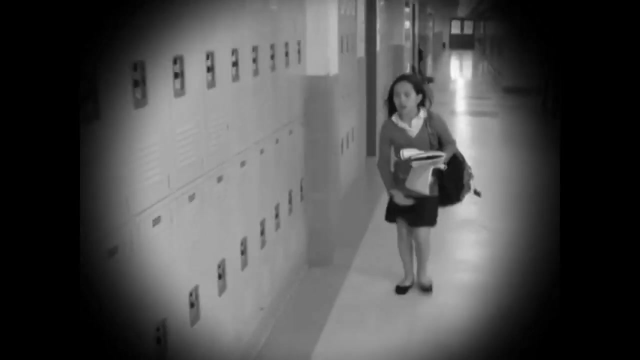 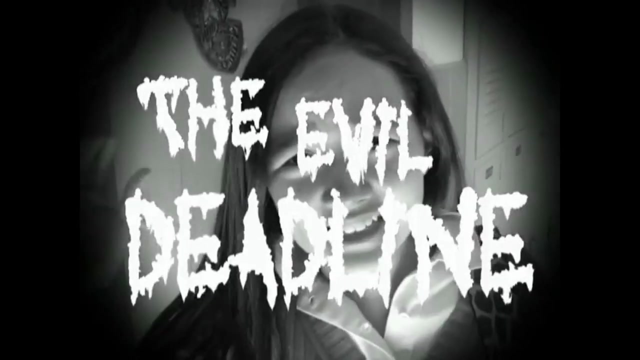 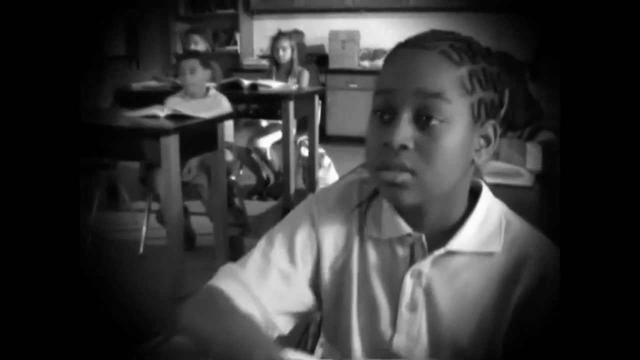 So, Paul, I forgot he had practice today. You're late- 500 push-ups. Laura left a homework to the last minute. I hope that everybody studied hard for their test today, And Ethan did. He did write down the day of his test. 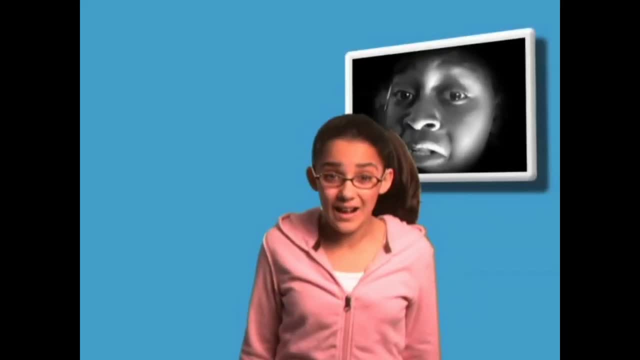 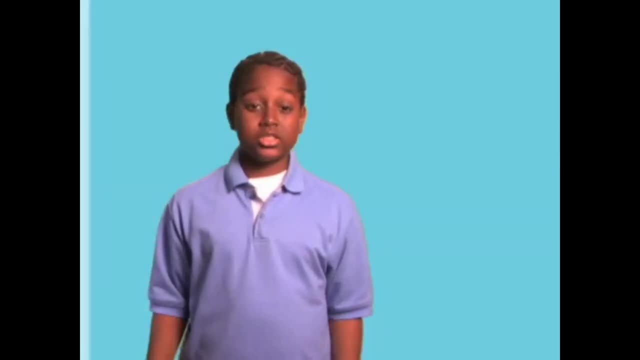 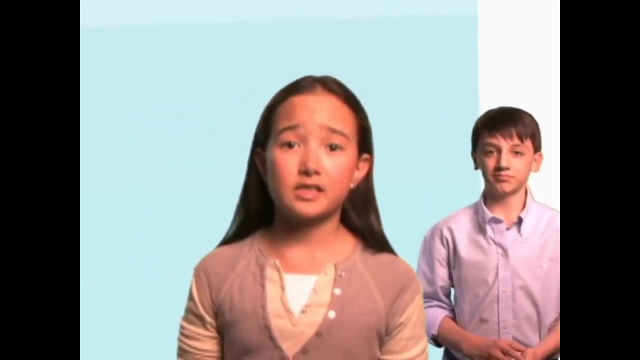 Wow, That was terrifying. I know Middle school can seem kind of scary anyway, and being disorganized just makes it worse. When I first started here I didn't know what to do. Everything was so different from elementary school: Lots of different subjects to keep track of, a bunch of teachers to get to know. 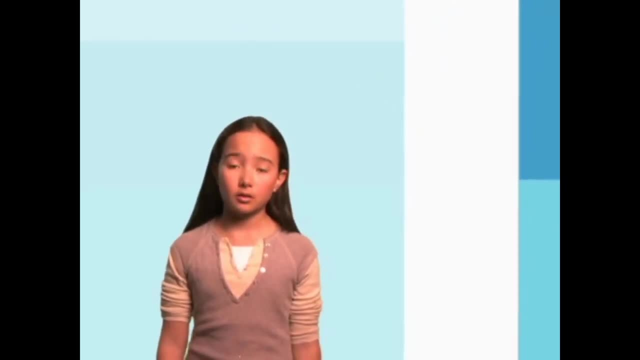 different rooms for each class. Everything about middle school was so confusing I felt the same way, But as soon as I got to middle school, I realized I was a bit confused. This is how it is in school. If you fail, this is how you fail. If you fail, you fail. I didn't know. If you fail, you fail. 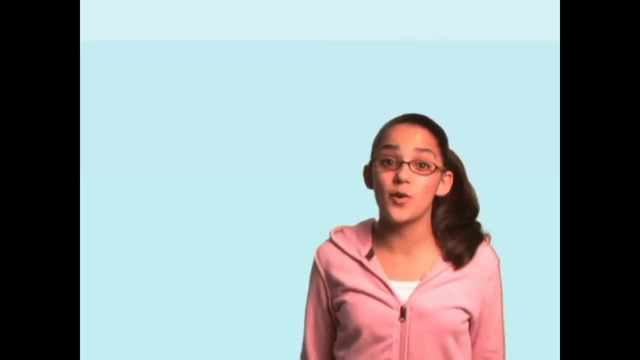 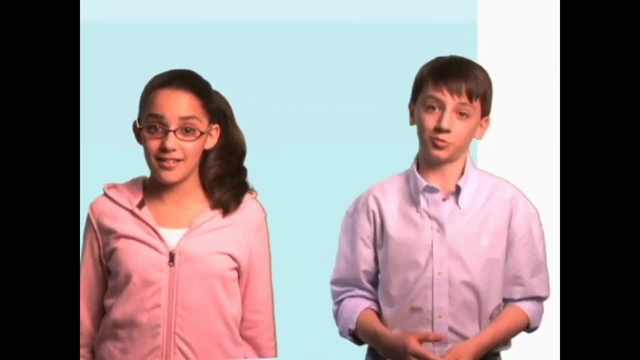 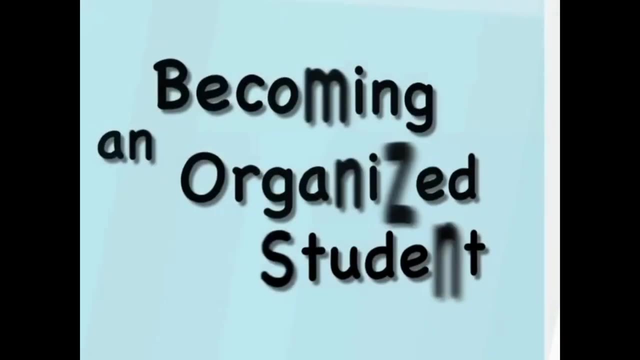 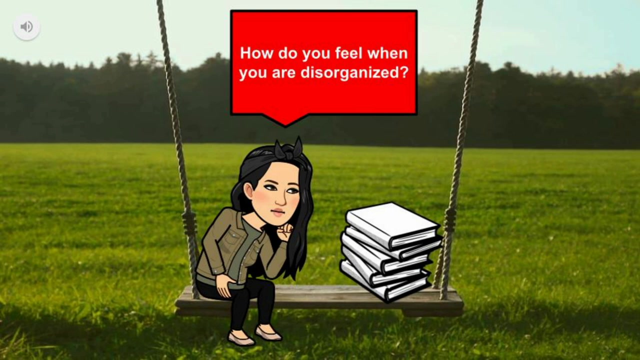 few simple strategies to stay on top of everything. Yeah, we all learn from our mistakes, And there were lots of them, And now we've got our act together. We know that being disorganized can be scary, stressful and not make us feel good. Think about how being disorganized makes you feel. 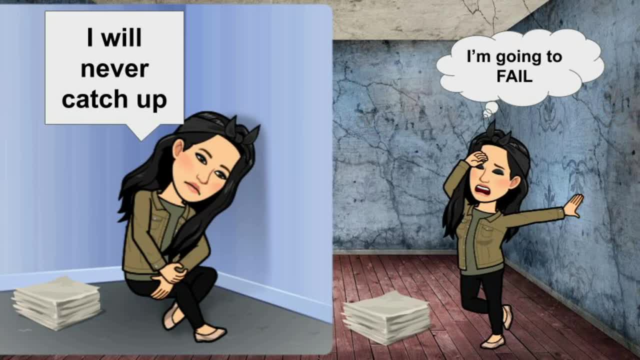 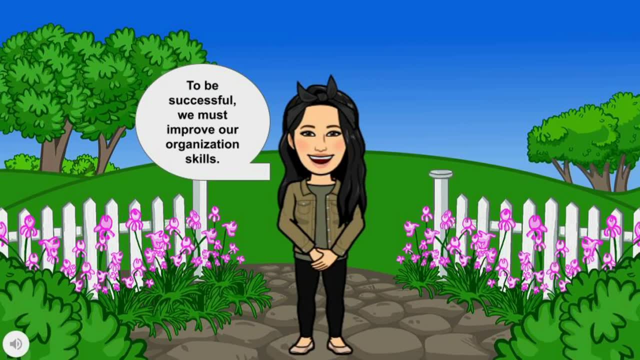 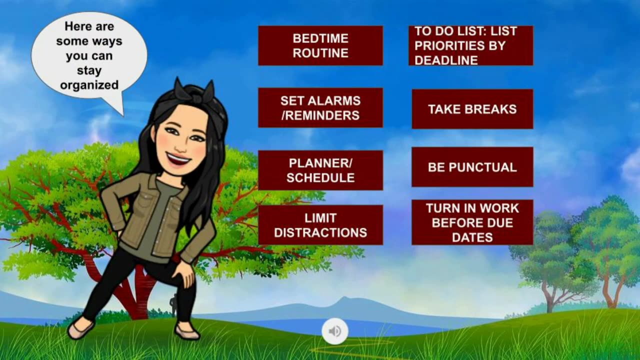 bad A lot of times. being disorganized can make us feel bad about ourselves too, Because we all want to succeed. we know that we need to work really hard to improve our organization skills. Here are some useful tips to help you be more organized. We can begin. 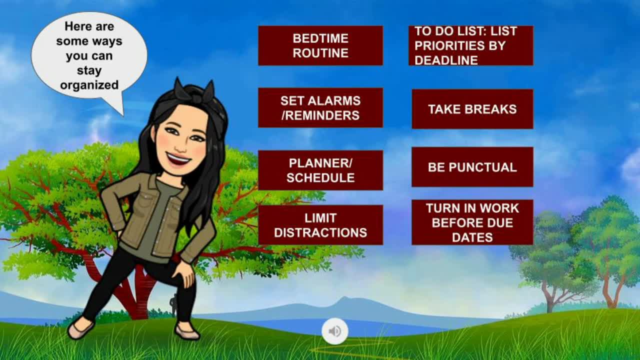 by establishing a bedtime routine. Think about what time you go to bed, What time do you wake up. Do you set an alarm, Maybe reminders to help you remember, Remember an important date? Having a planner, either a physical one or virtual one, can help you. 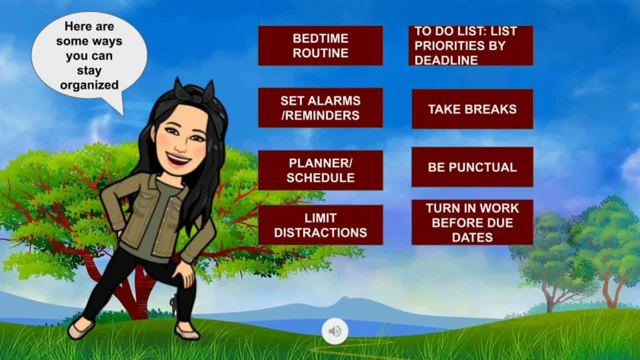 stay organized. Limiting distractions is also very important so that you are able to learn and focus on your work. Making a to-do list and checking it off as you go will help you feel very accomplished. Remembering to take breaks between tasks is very important. Always be punctual and 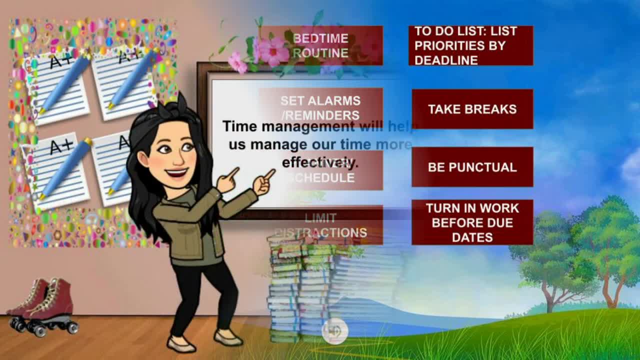 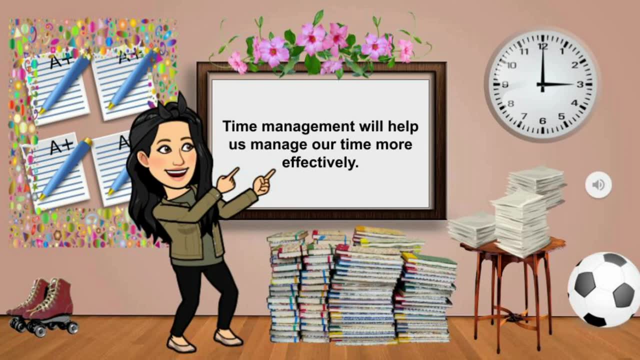 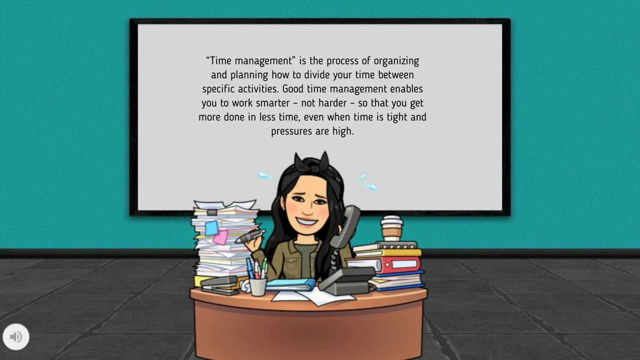 do turn in your homework before it is due. Now that you have learned about organization, I want to talk to you about Time Management. Do you know what that means? Time management is a process of organizing and planning how to divide your time between specific activities. Good time management enables you to work smarter, not harder, so 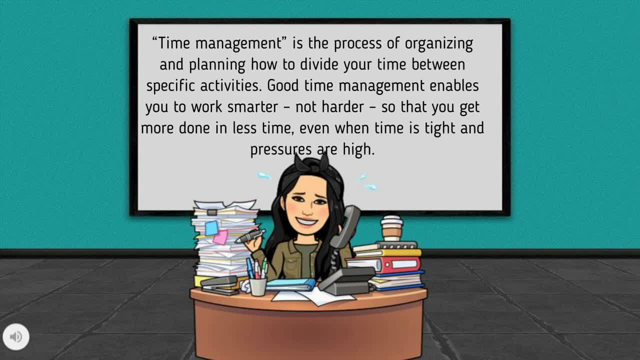 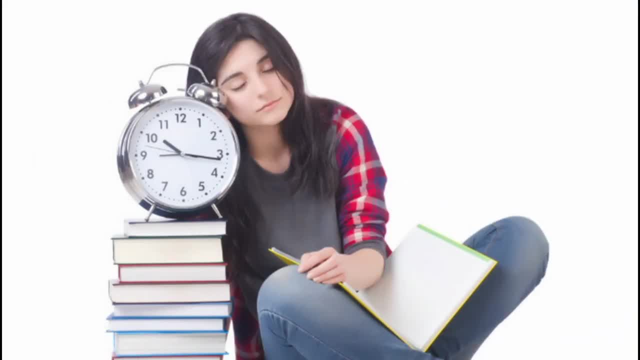 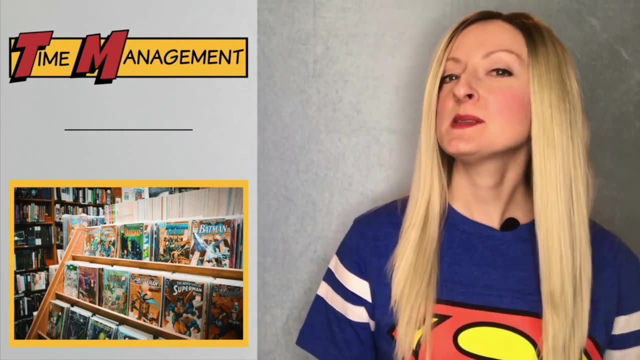 that you can get more done in less time, even when time is tight and pressures are high. But It's no advisable not to go. Nope, Part of being organized is learning to manage your time wisely. Which superhero comes to mind when I say time management? 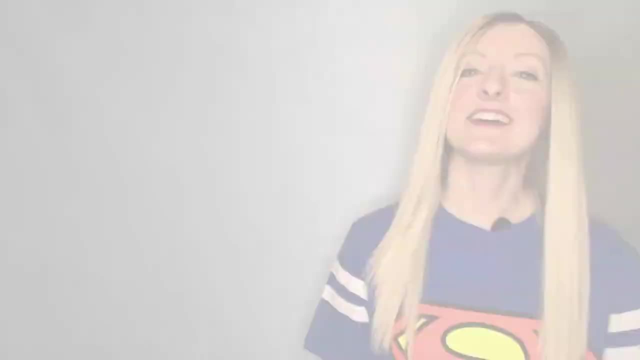 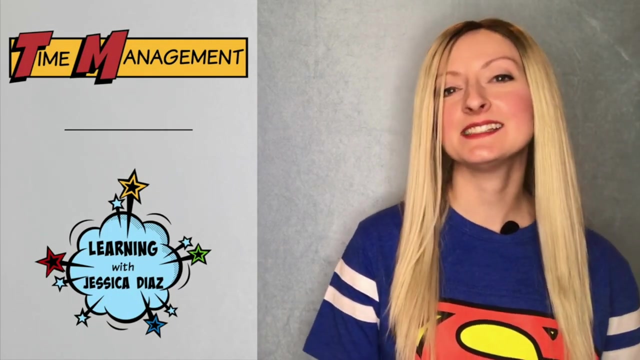 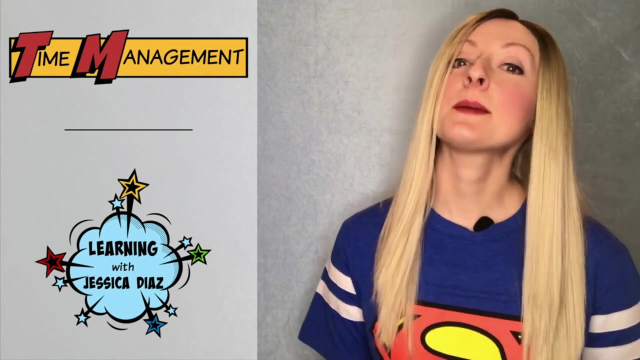 Is it Ant-Man? Maybe the Green Arrow? Let's find out. Hey, there I'm Jessica, from Learning with Jessica Diaz. So before we can decide which superhero has the best potential for great time management, let's talk about what time management is and how we can be better at it. 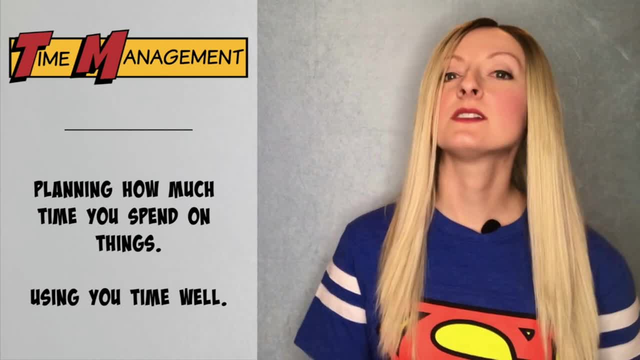 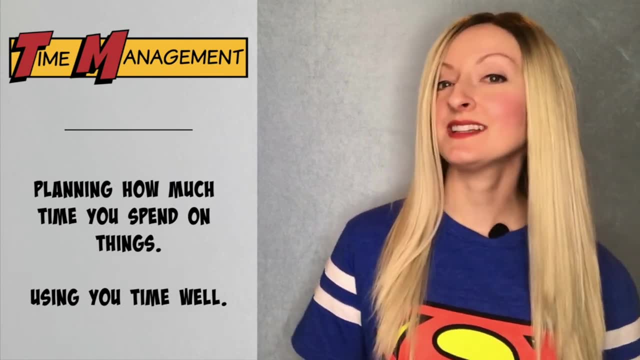 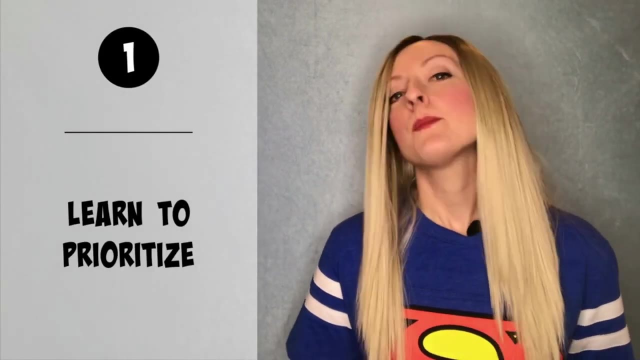 Time management is planning how much time you spend on certain things. It basically boils down to spending your time well, Wondering how you can manage your time more effectively. Just keep these three things in mind. Number one: learn to prioritize. Prioritizing means that you can figure out what's most important and do that first. 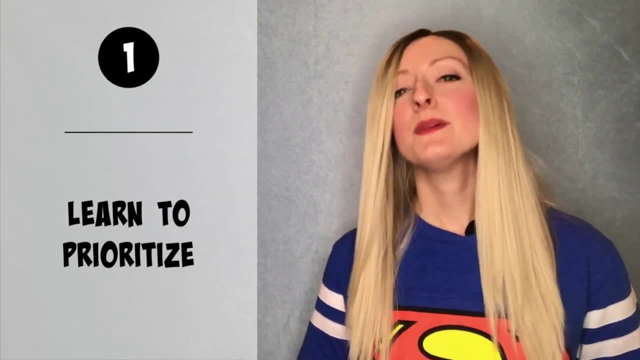 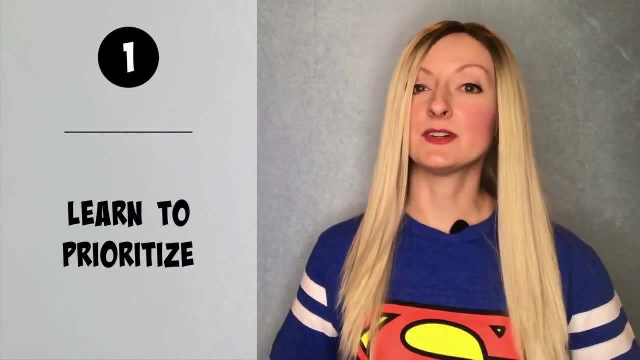 So let's say that you need to clean your room and do your homework, But you also really want to play Luigi's Mansion 3.. Well, if you're prioritizing, you'll do the most important task first, followed by the task that's next in line at being the most important. 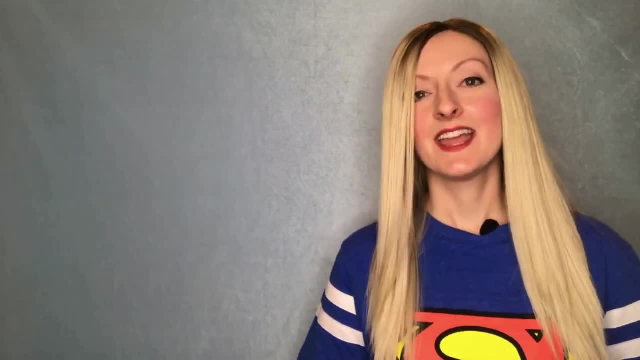 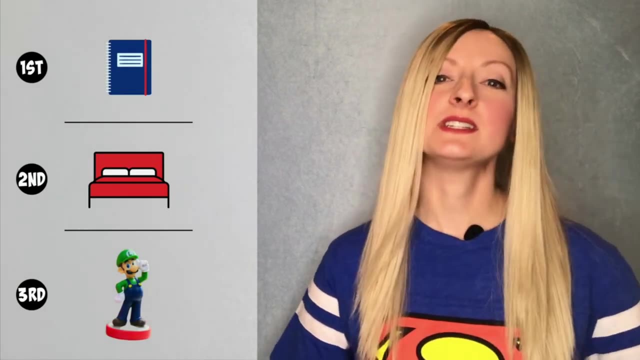 And that you can save time for fun stuff once you're done. So if I were prioritizing these three things, I would do my homework, then clean my room and then play Luigi's Mansion 3.. Number two: make a to-do list. 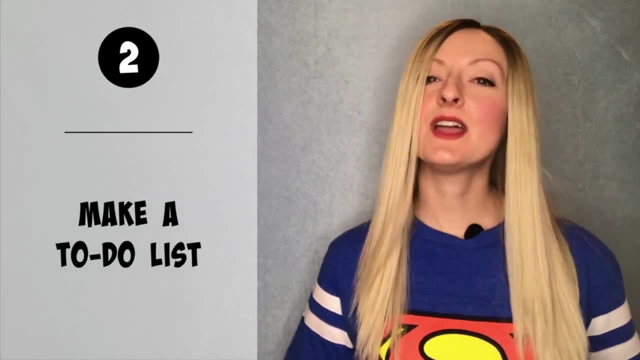 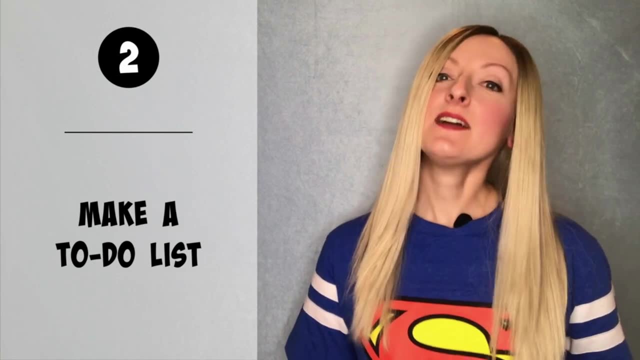 A to-do list is just a list of things that need to get done. Now. if you're new to making to-do lists, it can be helpful to ask an adult for help, But it basically looks like this: Let's say that I have homework chores: taekwondo practice. 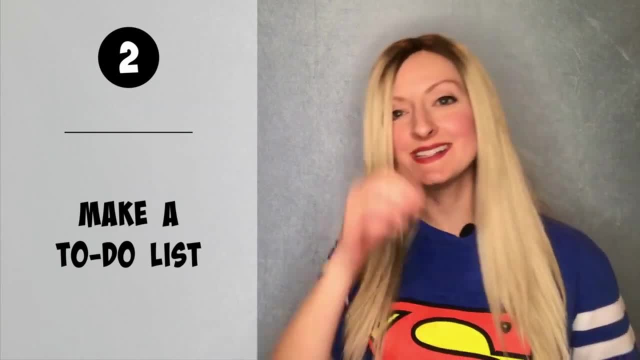 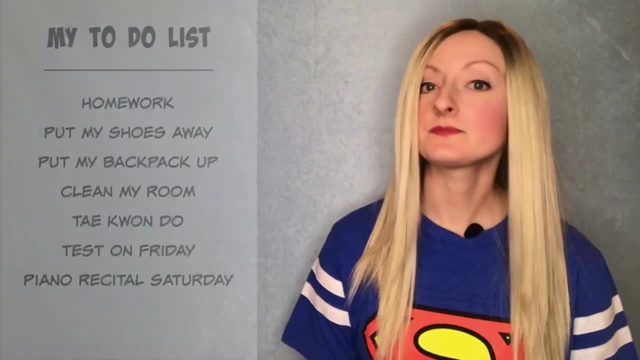 a test coming up on Friday and a piano recital on Saturday. That's a lot to keep track of And I'm worried that I might forget something, So I write it all down: The homework, putting my shoes and backpack away. 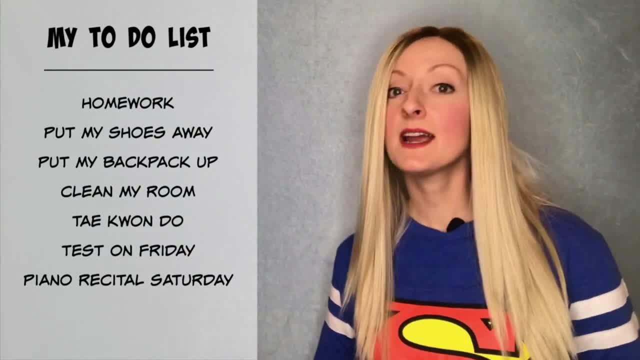 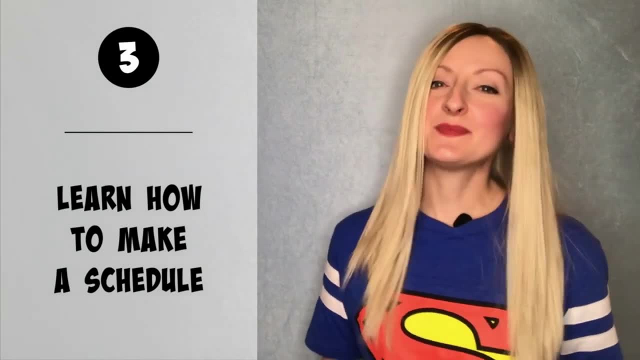 the cleaning my room. taekwondo practice my test on Friday and my piano recital on Saturday. Number three: learn how to make a schedule. A schedule is just a plan for when you're going to do things, So if you know that you're going to have a test on Friday, 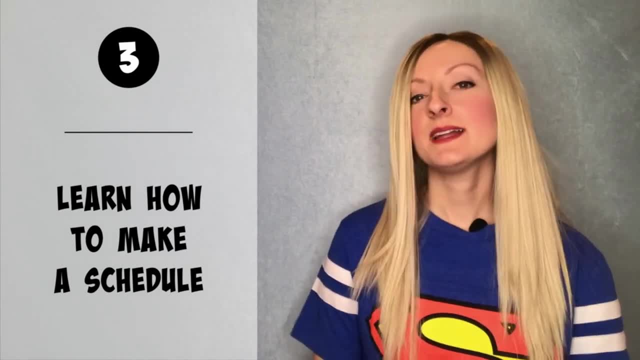 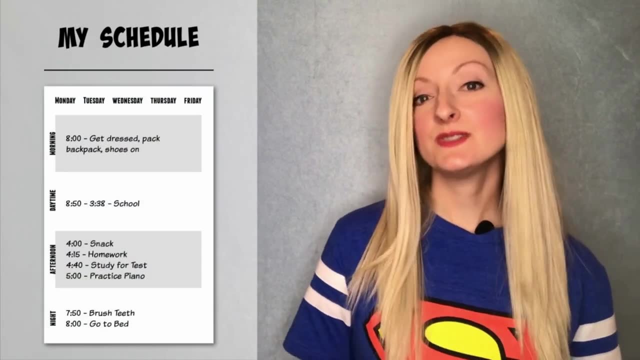 and a piano recital on Saturday. you might plan to set aside 20 minutes each night to study for your test and to practice playing the piano. If you write your schedule down, it might look a little something like this: Okay, now you're ready, right. 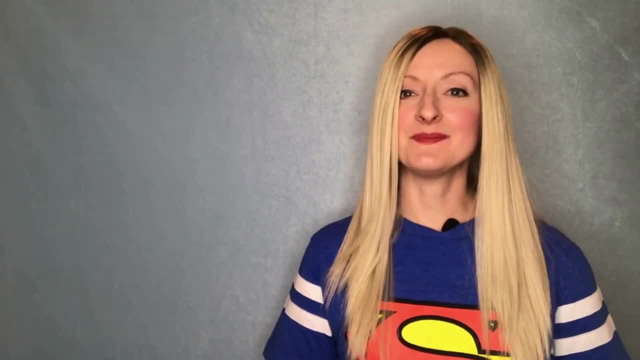 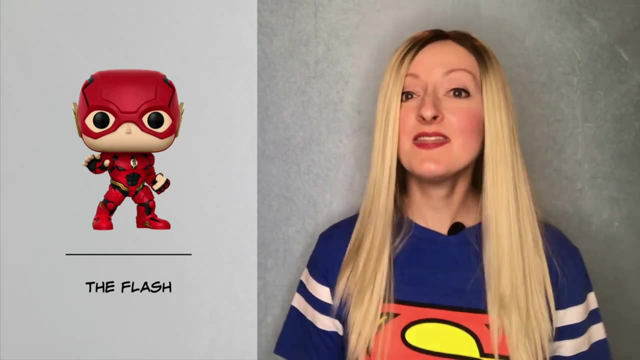 You're ready to know which superhero has the best potential for time management. It's the Flash Duh, right? Can't you imagine having that super speed? How quickly you get things done. Homework- two seconds done. Chores- three seconds done.